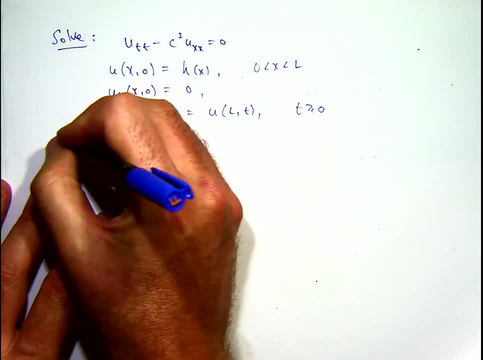 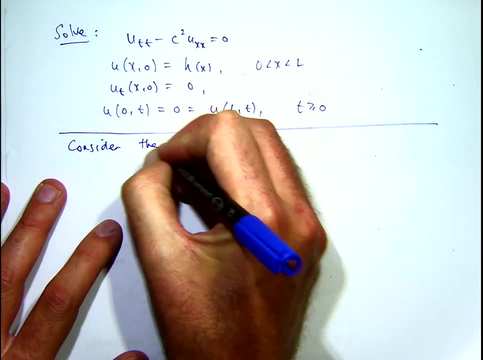 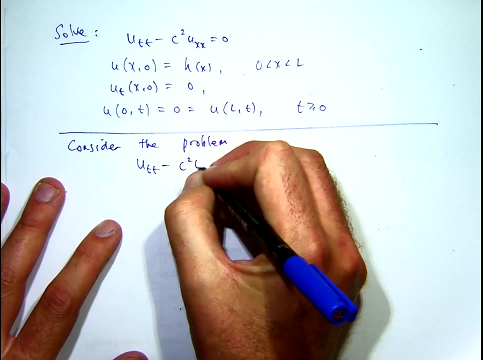 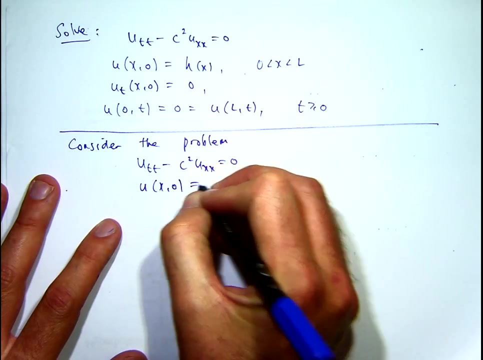 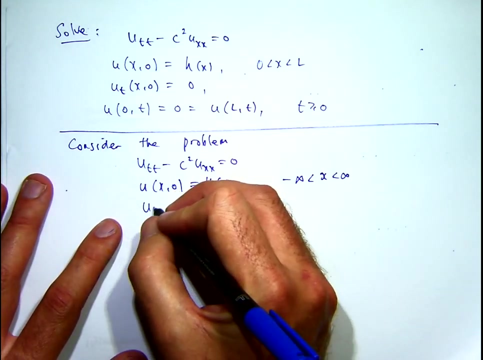 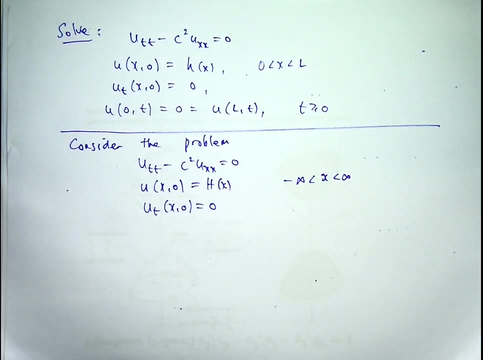 So we'll come back to that. So just something quickly about d'Alembert's solution. Okay, so let's consider the related problem Now. essentially we're going to relate big H to little h, But let's just consider the second problem independently of the first, for now, 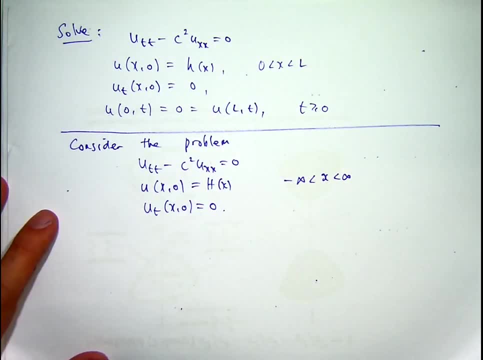 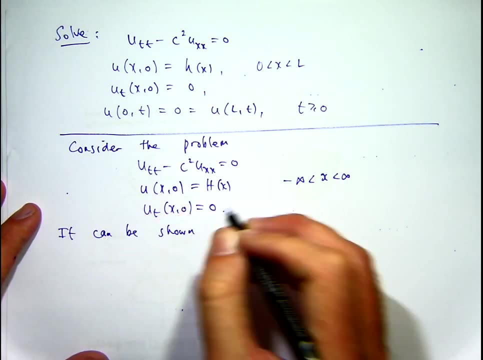 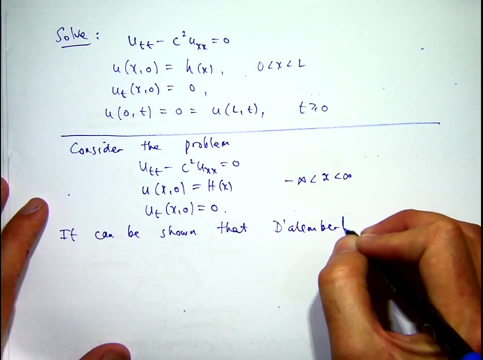 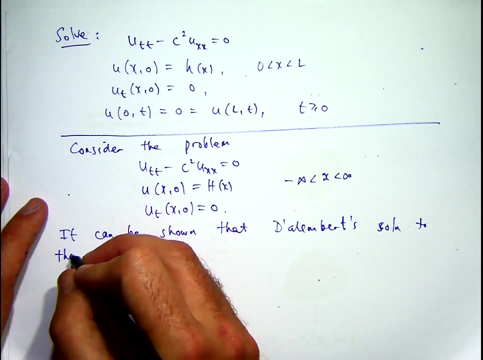 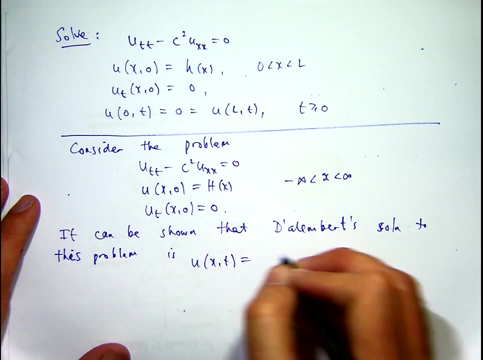 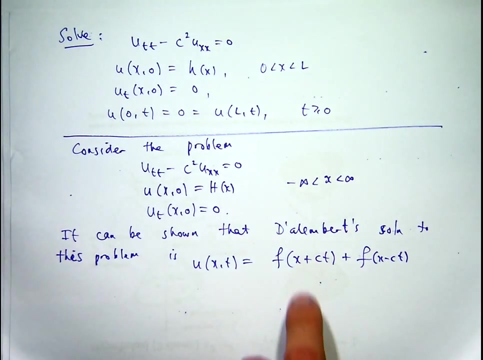 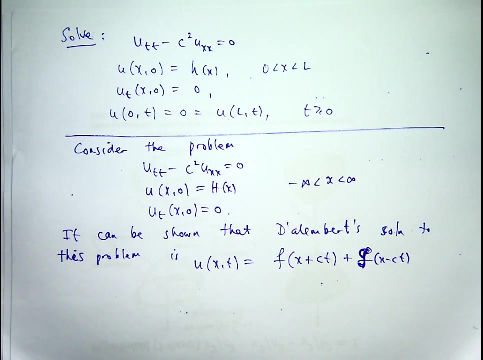 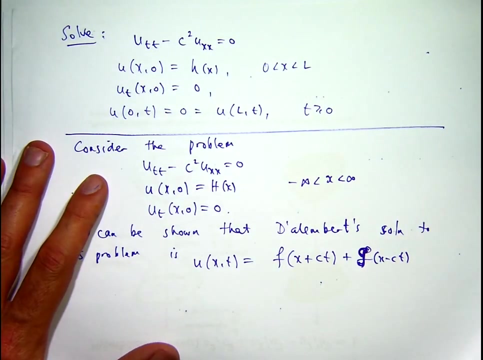 Okay, It can be shown that d'Alembert's solution to this second problem is the following: Okay, In fact we've verified that in another video, another presentation, where f and g are just twice differentiable functions. Now, in fact, you can go a bit further and actually say that you can relate these two functions with the initial displacement. 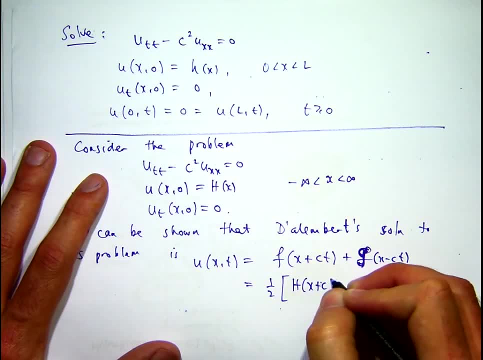 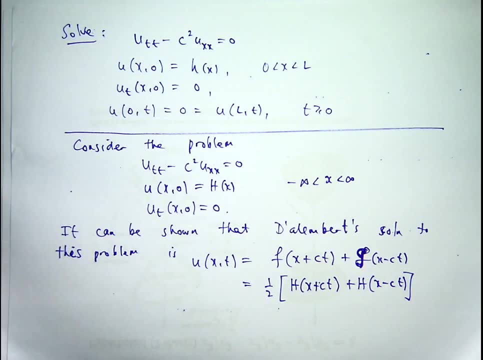 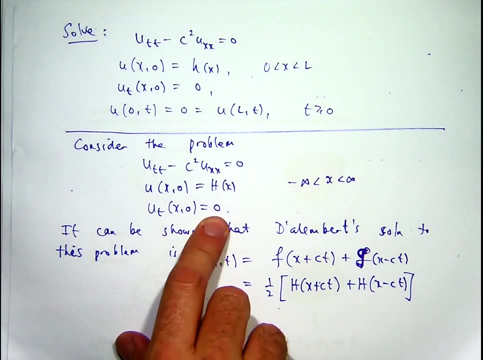 Okay, So we'll come back to that in a minute. Okay, well, how do you do that? Well, Don't you also have an integral now like that? No, because the Yeah, you would have, You would. 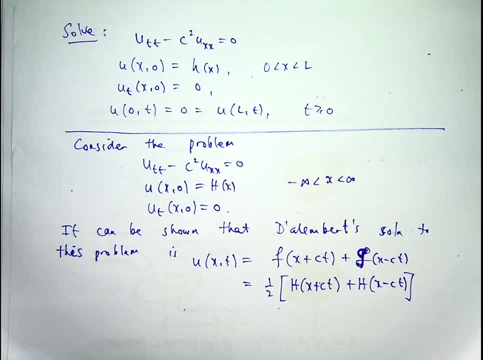 If that was a function, definitely Yeah. if that was non-zero, you'd definitely have an integral, Okay. So how do you come up with this? Well, essentially you use these two conditions, Okay. So the first condition it'll be: h of x equals f of x plus g of x. 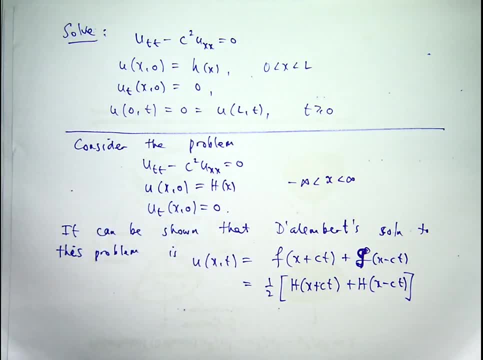 Okay, The second condition will be something like: cf dash of x minus cg dash of x equals zero, And if you differentiate the one involving h of x, Then you can actually go through and determine f in terms of big H and g in terms of big H. 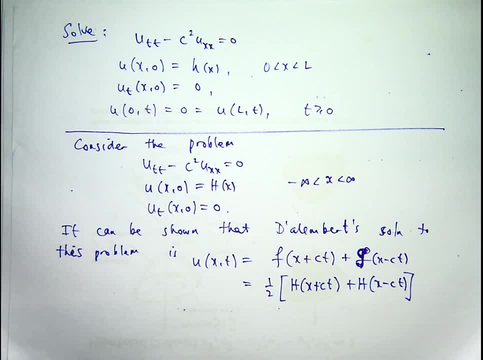 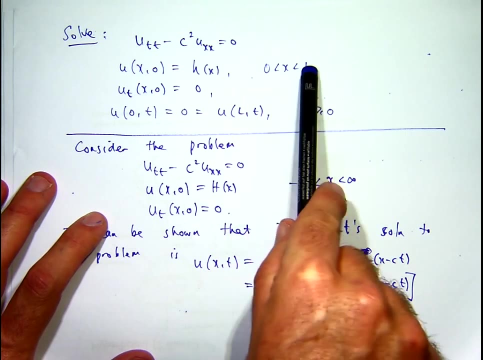 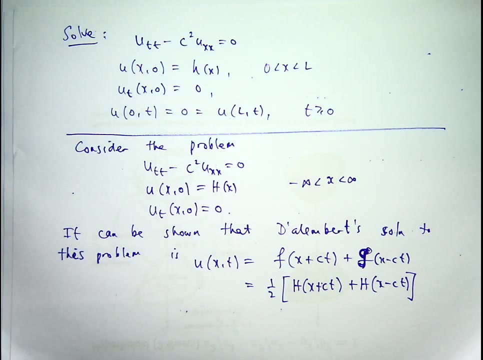 Okay, All right. so how can we use this to actually solve the original problem? Well, this initial pluck, or initial displacement is only defined on this interval, Whereas this is defined on the whole real line. So what we're going to do here is actually extend little h to the whole real line, but in a very clever way. 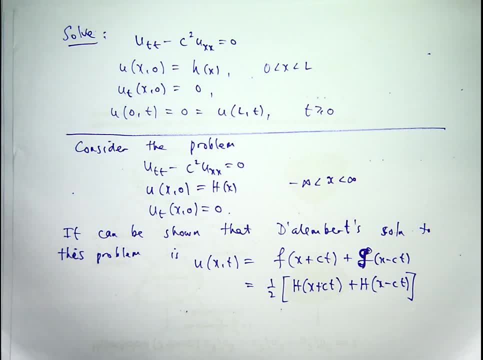 Okay, We're going to extend little h as an odd periodic function. Okay, You might think: well, why? Why do you want it? Why that? Why not something else? Why not an even function? Why something like that at all? 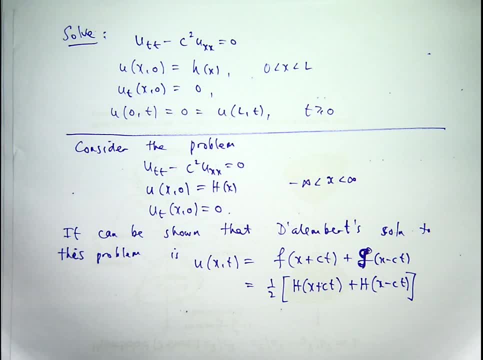 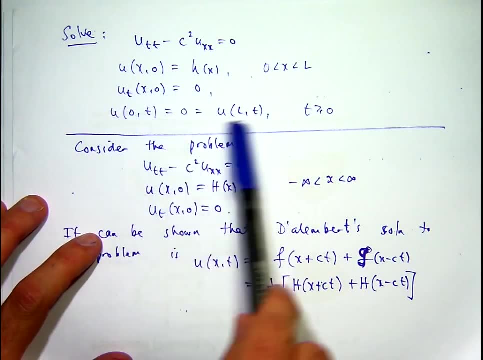 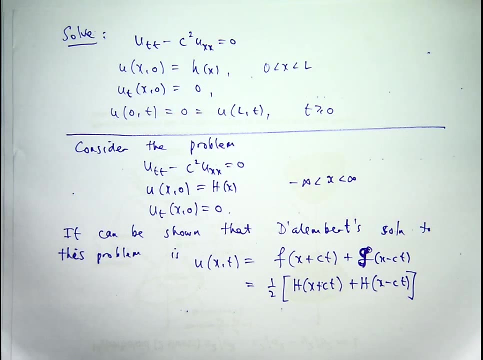 Well, it'll become clear why these things work as we actually verify That these. Essentially, it's about verifying that these two conditions hold Okay, And you'll see where we use the concept of periodicity with period 2L and the oddness. 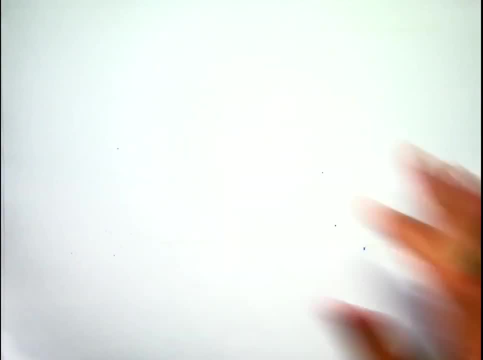 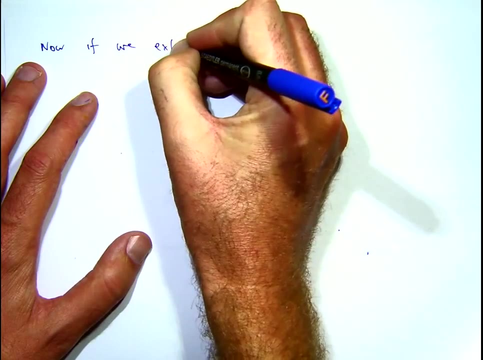 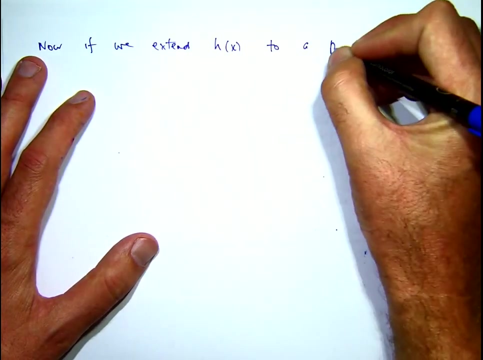 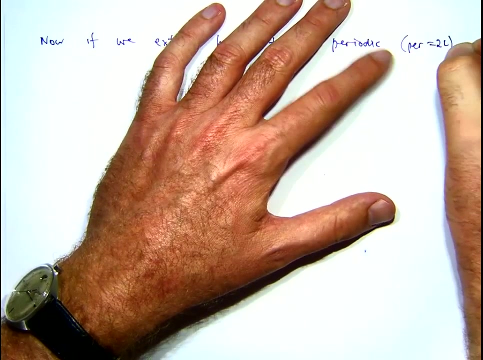 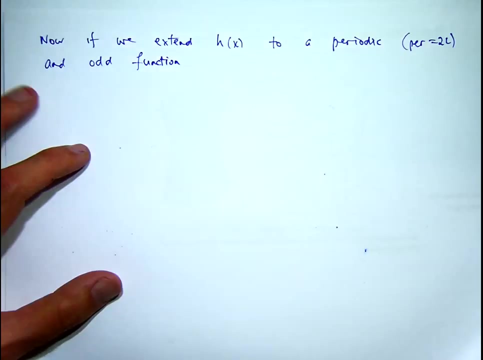 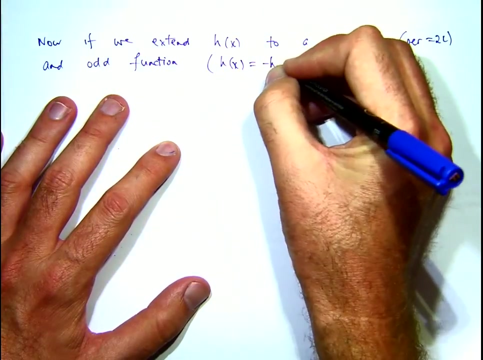 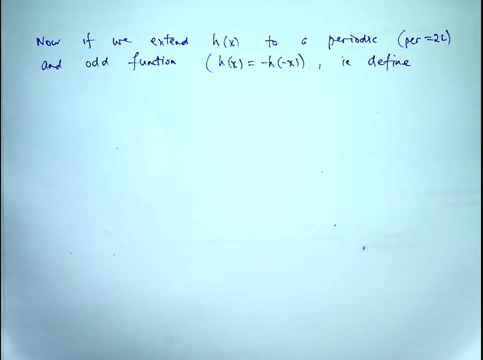 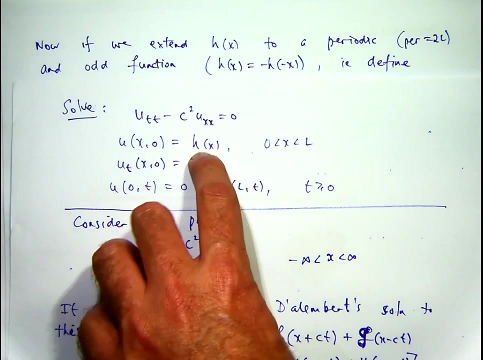 Okay, So that's our goal. So that's, That's a very simple function. Okay, a periodic, An odd function. So You're going to define this function here and relate it to so big H is going to be the odd periodic extension of little h. 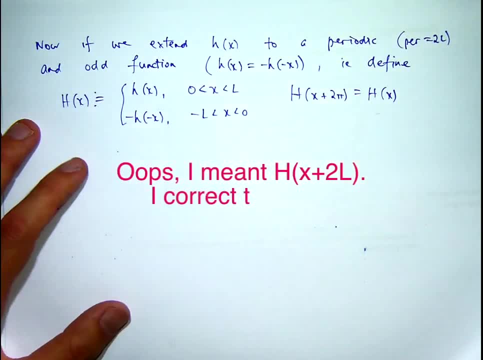 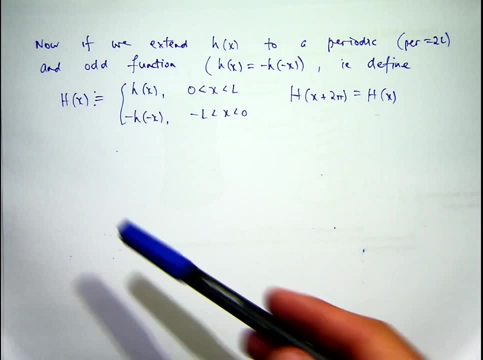 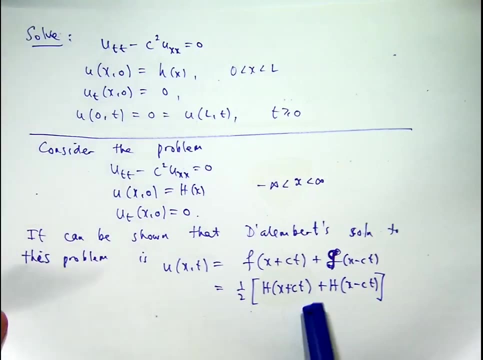 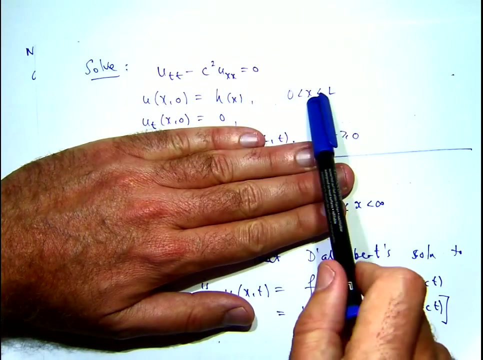 then we already know that this problem has a solution of this form. so what we've done is we've taken something that's not quite defined, or this thing that's not quite defined on the whole real x, we've extended its domain of definition, and we've extended its domain of definition. 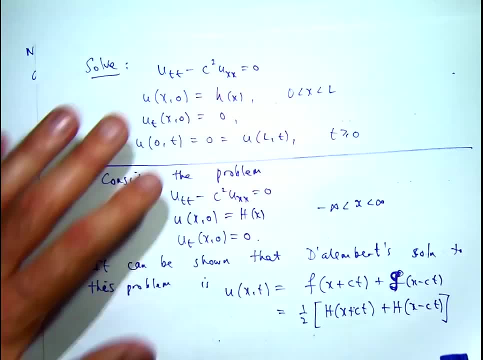 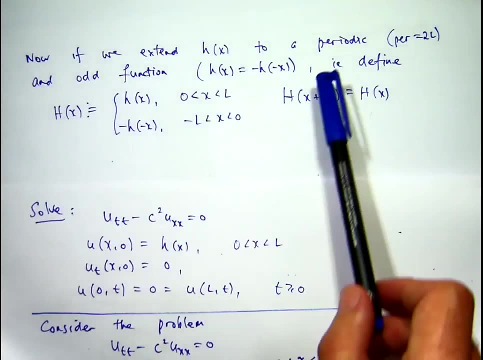 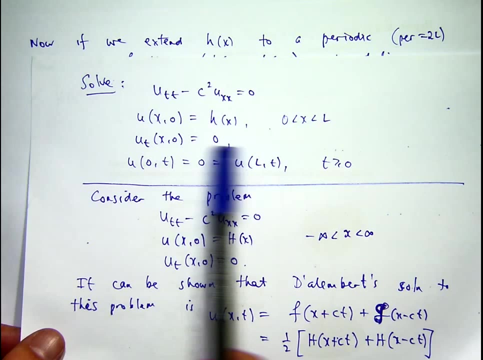 and we've extended its domain of definition in a certain way, and we know that that problem has a solution of this form. so now what we want to do? notice: we haven't used any periodicity or any oddness of this extension. yet the oddness and the periodicity comes in with satisfying these conditions. 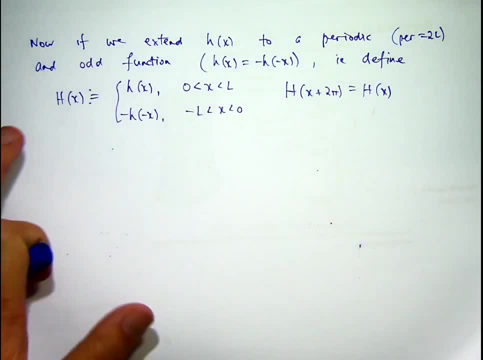 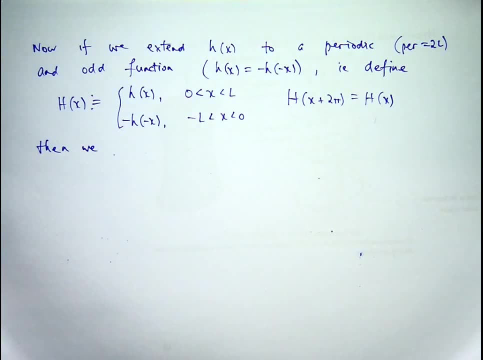 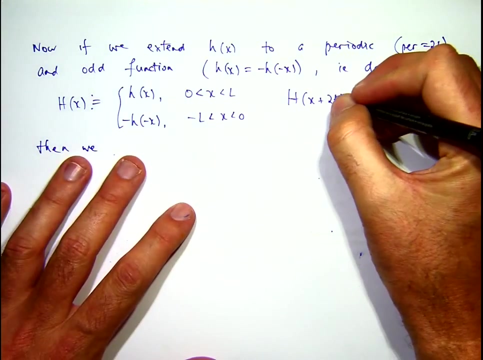 the side conditions or the boundary conditions. ok, is it H? x plus the capital, H x plus 2 pi or x plus 2L? oh, 2L, yeah, thank you, so that's 2L. I've got Fourier series on the brain. 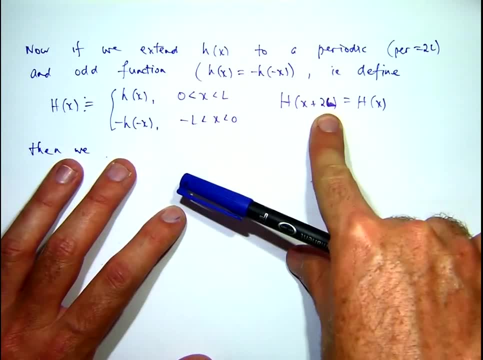 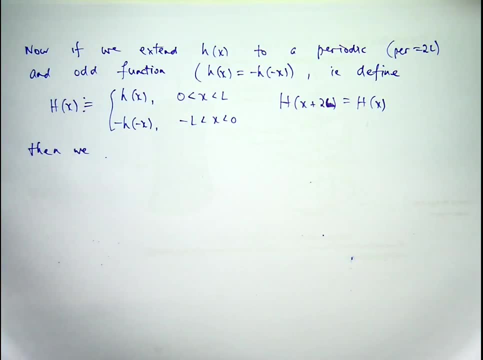 ok, so it's not 2 pi, sorry, 2L here. thank you, ok, 2L. yeah, Fourier series with 2 pi periodicity. they're a hard thing to ignore. ok, so 2L. thank you for that. 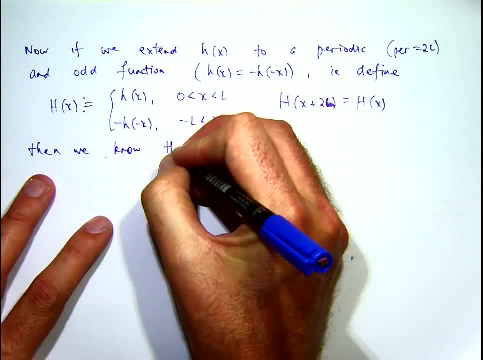 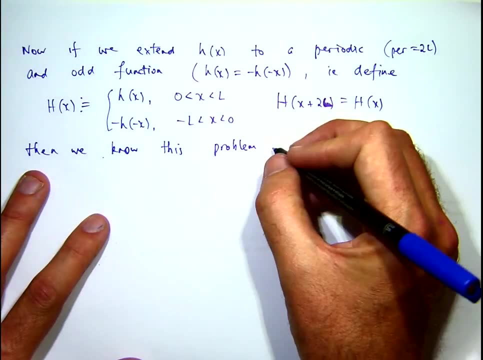 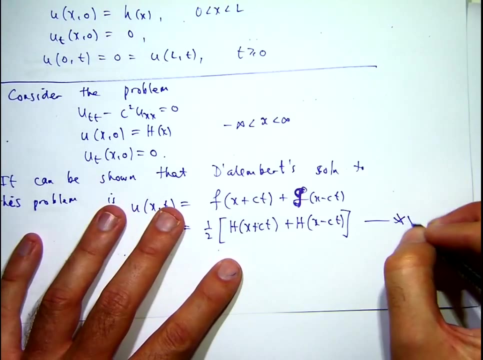 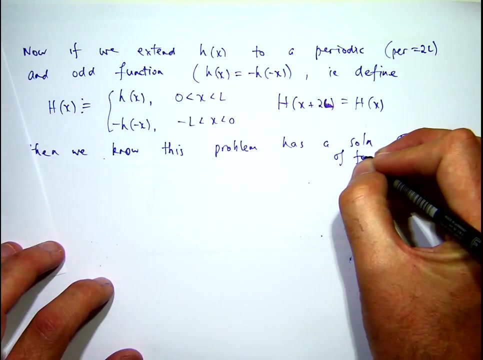 then we've got 2L, ok, so 2L, thank you for that. then we know this problem has a solution and the solution, say, is in double star, form of form, double star, ok. so now what we want to do. 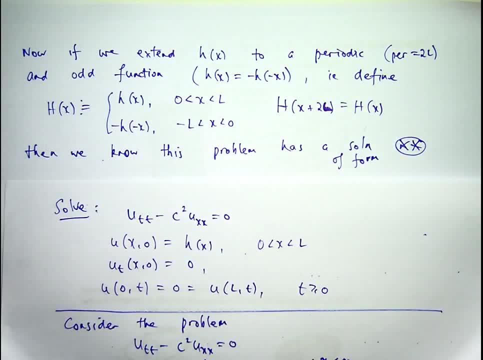 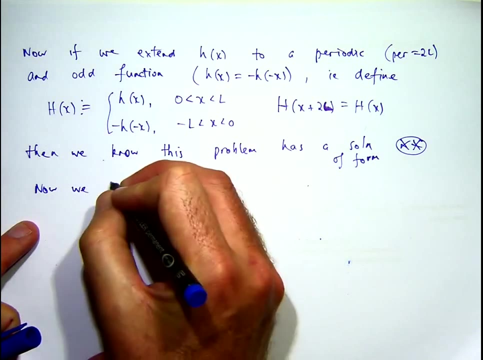 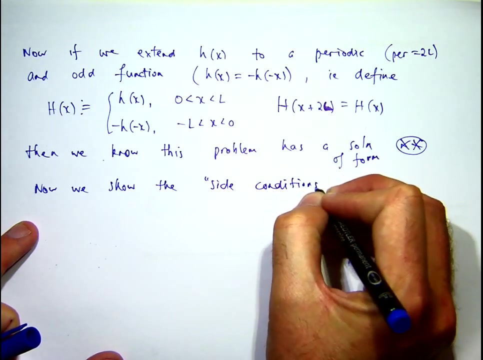 is actually show that if our periodic extension, our periodic extension, our odd extension, essentially gives us these, the boundary conditions, the zero side conditions. ok, so, as a final step, so I'm going to call these side conditions. so let's call, let's make that S. 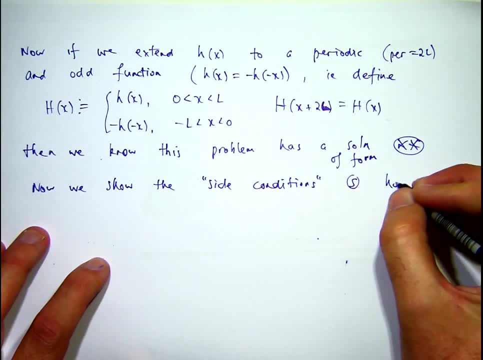 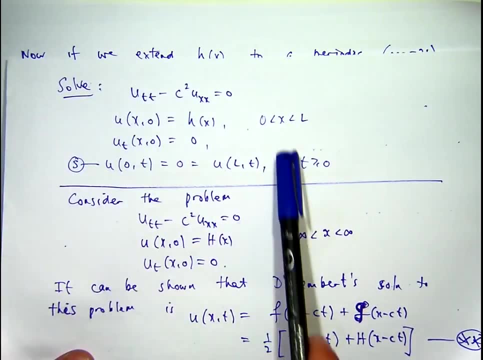 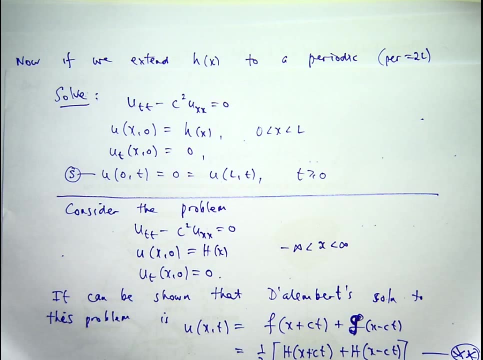 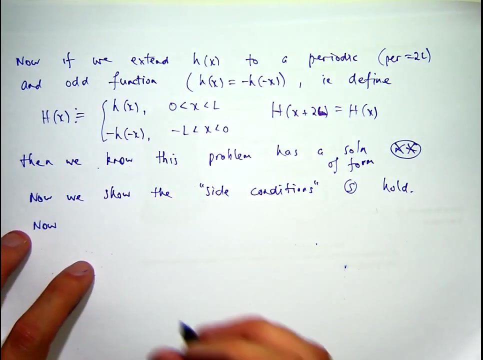 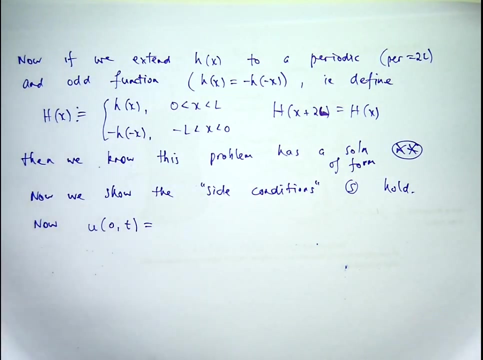 S for side condition. ok, because what that means is? it means that the solution of this form must satisfy the original problem, or you know, for X, between 0 and L and all T, positive or non-negative. ok, alright, so Let's set this for the binomial. 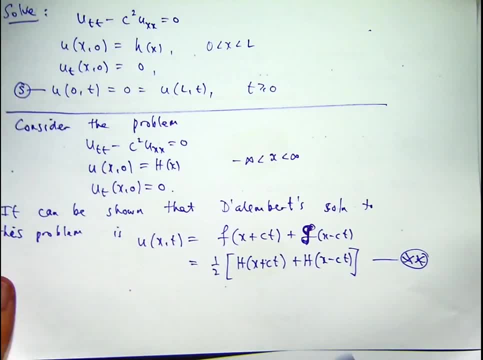 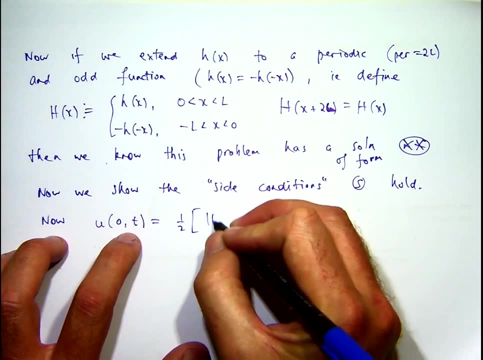 ok, so I'm going to do this, so it's going to be so. using this, where H is the odd periodic extension, big H is the odd periodic extension of little H. let's show that this equals zero. ok, so if you go in and plug in, X equals zero. 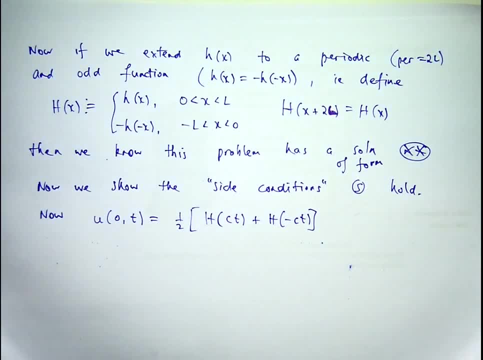 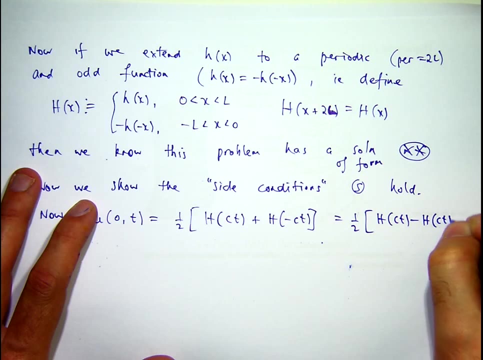 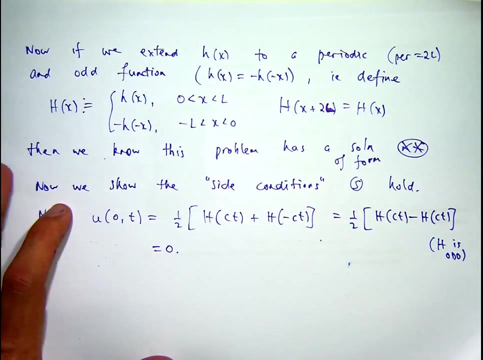 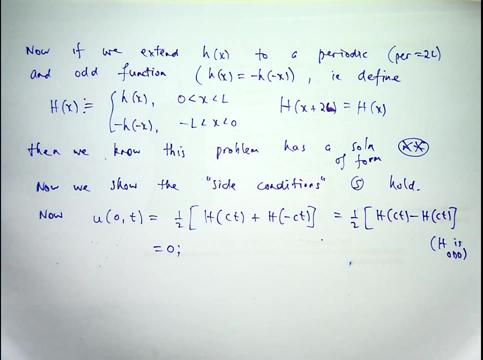 you'll get the following: now, what we want is these terms to disappear, cancel each other out, and we know they do, because we've assumed that big H is odd, ok, So what do we get here? We get zero, Nice. So, in other words, this solution satisfies the left side condition. 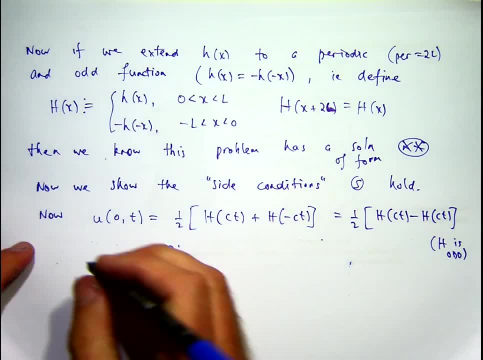 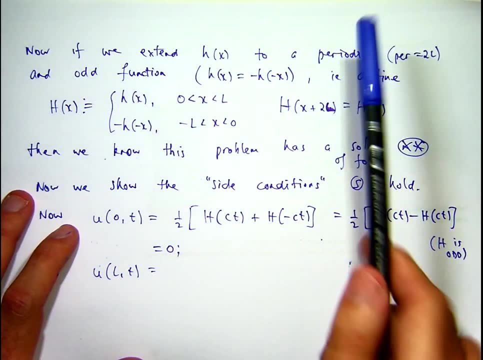 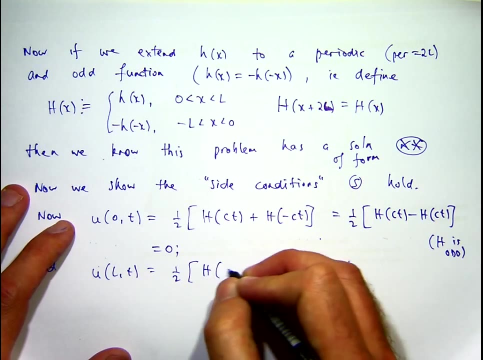 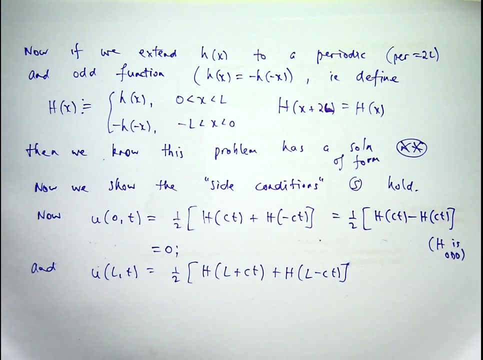 if you like. What about the other side condition? Well, we've used the oddness, We haven't used the periodicity yet. So if I go back to double star and plug in x equals capital L, I'll get something like this: 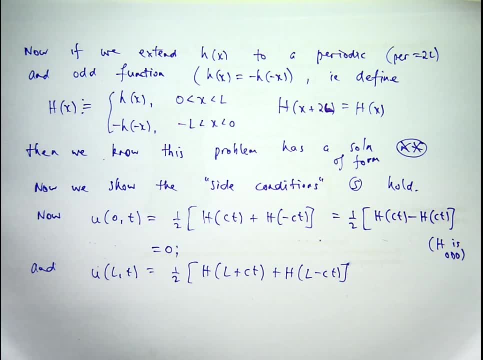 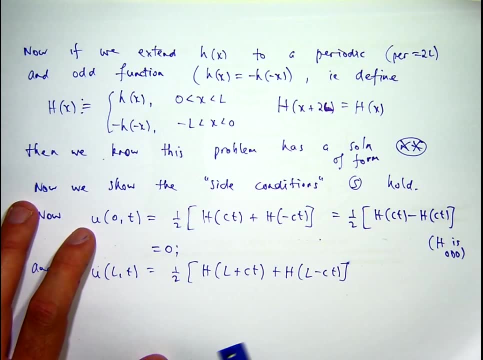 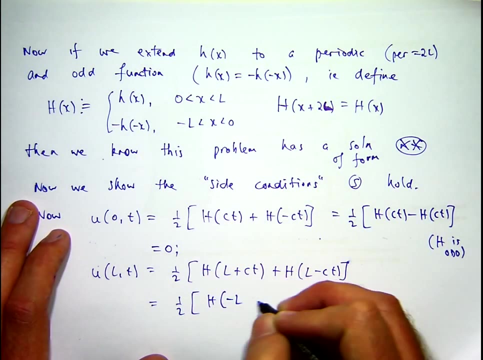 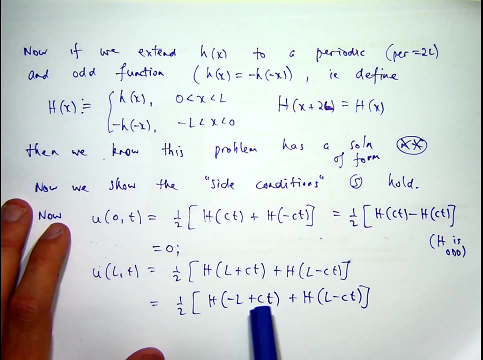 Now we want these two things to cancel each other out in some sense. So how do we do that? Well, h is 2 pi, periodic big H. So certainly this is true And this is the negative of that. So, if I use the oddness, 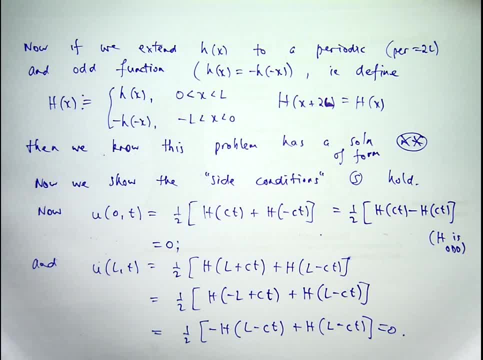 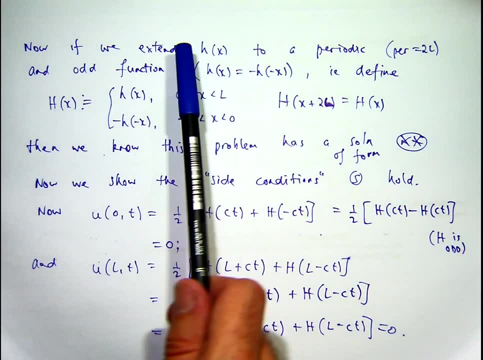